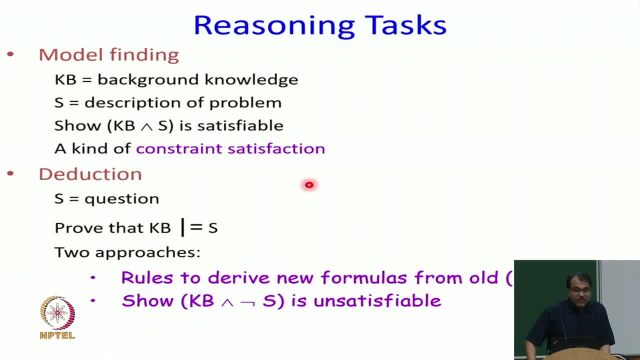 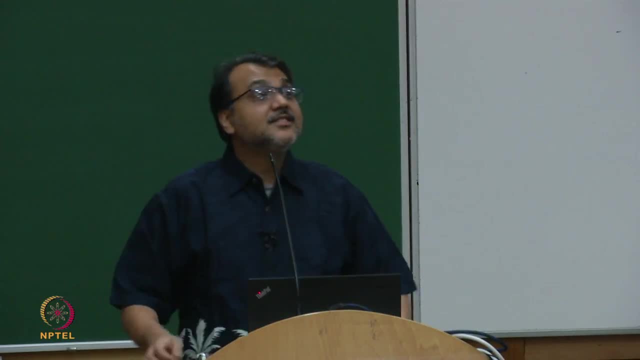 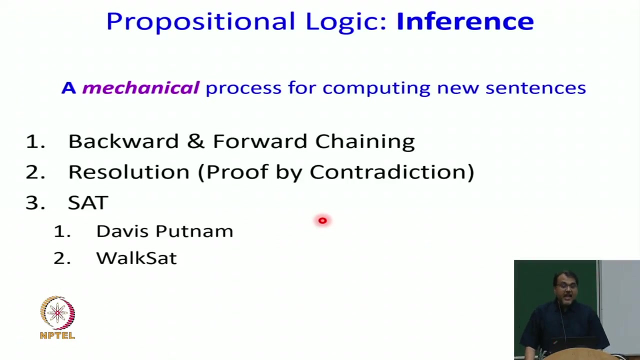 do this? Prove by contradiction. So this style of proving KB and not S unsatisfiable is equivalent to mimicking proof by contradiction. So now we are getting closer to our first inference algorithm. Now, what is an inference algorithm? It is a mechanical process for computing new sentences, and we will study. 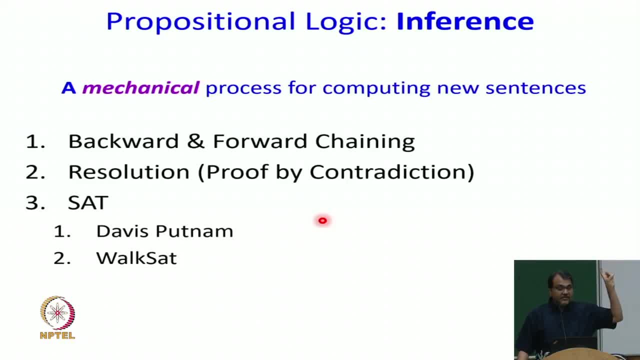 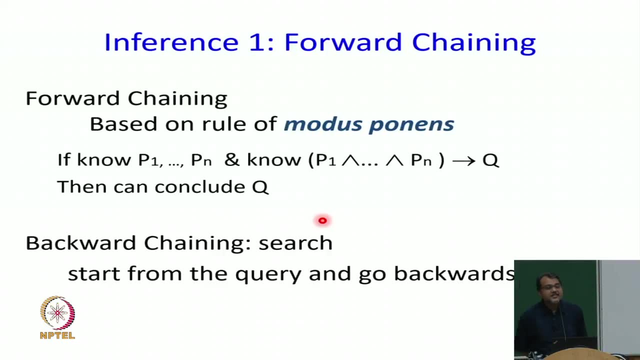 three of them: Backward and forward chaining resolution, which is equivalent to proof by contradiction, and three satisfiability problem, which is equivalent to model checking, model finding. So let us look at the very first one, The first simple inference procedure, and that is called the forward checking procedure. 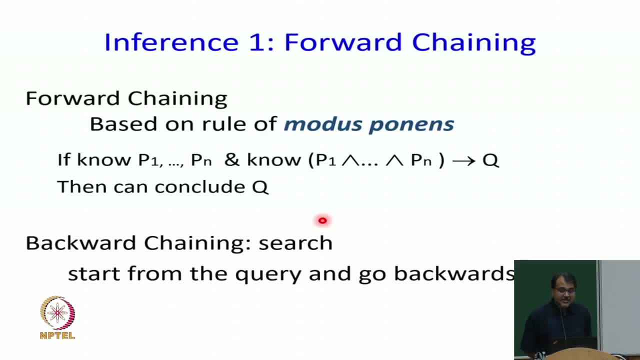 The forward checking is based on the rule of modus ponens. Modus ponens basically says, if I know, P1 and P2 and Pn imply Q, and I also know that P1 is true, P2 is true and Pn is. 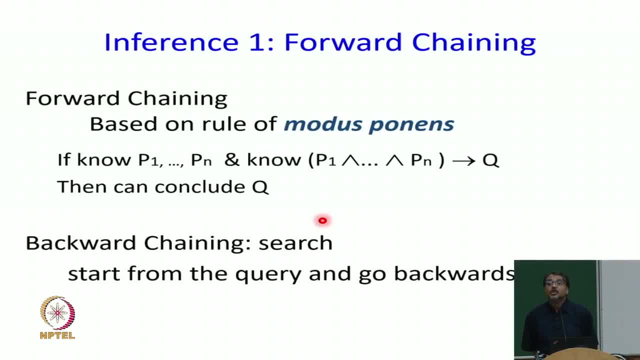 true, then I can prove Q to be true. It is as simple a rule as that. A and B comma. A implies B, A implies B and A implies B. Okay, Okay, This is how you will accurately say it in the language of logic: that in any world, in 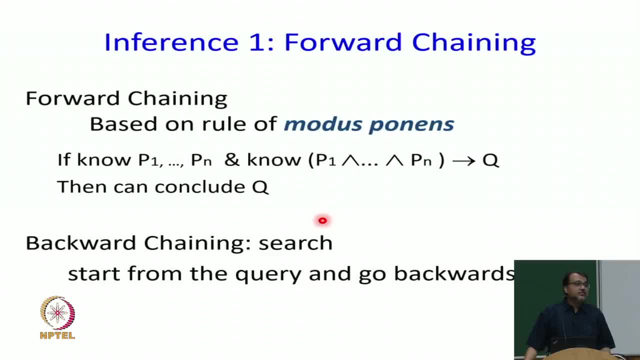 which A implies B and A is true, then B is true. Now this rule, if you apply appropriately and prove new things, this is called forward chaining. I am starting with what I know and using this rule to prove new things in the future. 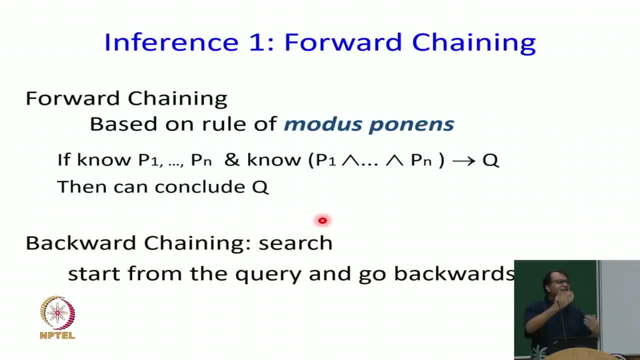 So I am going to prove new things in the forward direction. There is always a backward version of things, like you had forward search, you had backward search and then you had bidirectional search. The same way, backward chaining says that there is something I need to prove. Now let me see. 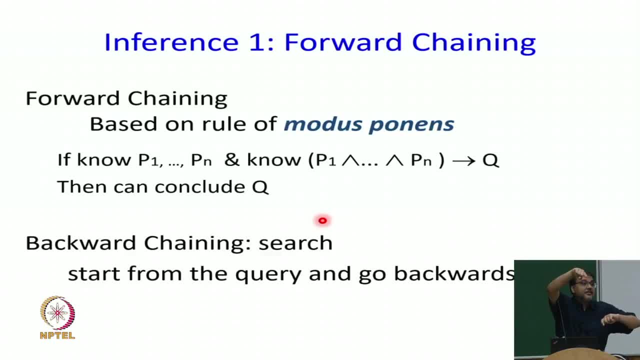 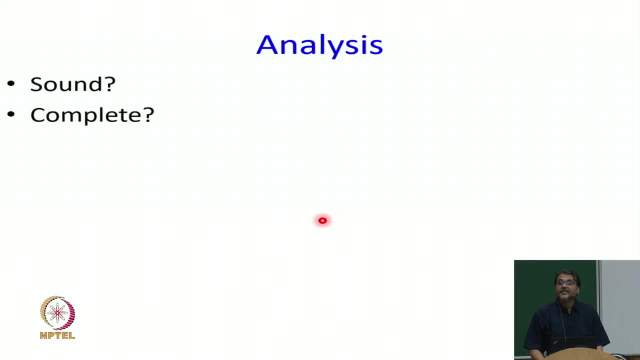 what thing should I have had in my knowledge base to be able to prove it? And then let me see how I can prove these things, and I keep going back, and that is called backward chaining, Anyway. So if I only do modus ponens in the forward direction, would it be a sound procedure? 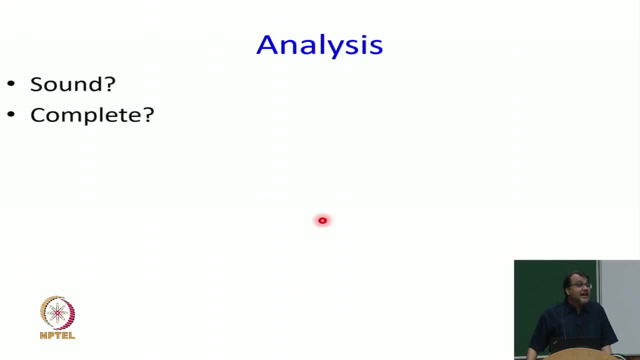 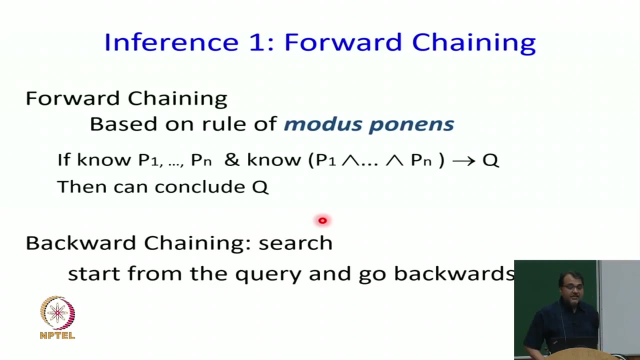 Whenever I apply modus ponens and prove a new thing, will it actually be entailed? Come on, this is not a very hard question. So the question is if this is the only rule I was applying that whenever I know P1 to Pn, and I also know that P1 to Pn implies Q and therefore 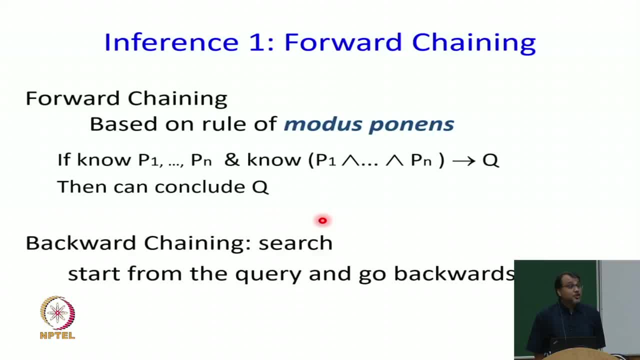 based on this knowledge, I prove that Q is true. I know that P1 to Pn implies Q and therefore, based on this knowledge, I prove that Q is true. I know that P1 to Pn implies Q and therefore, based on this knowledge, I prove that Q is true. Will Q really be true? Yes, 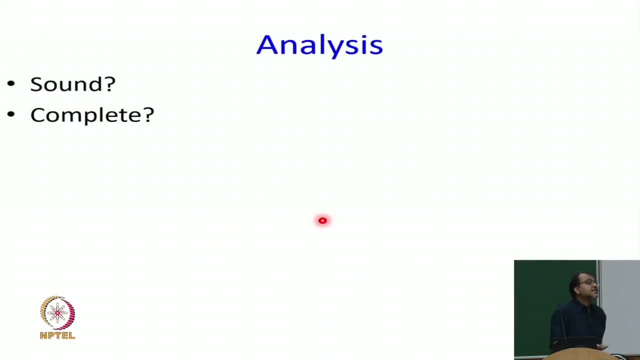 So will it be a sound algorithm? Yes, it will never say something which is incorrect. Will it be a complete algorithm? Will it be able to prove everything that is true? Can you give me an example? It will take you some time to think about it, But I will give you. 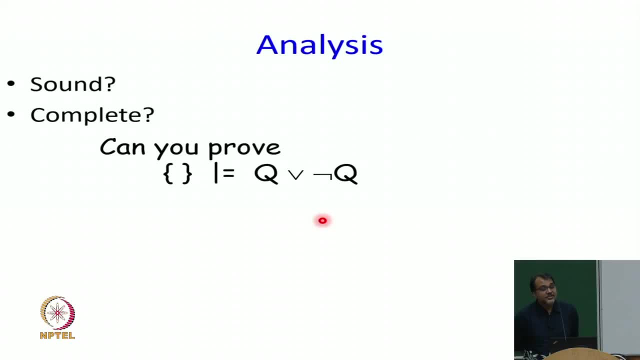 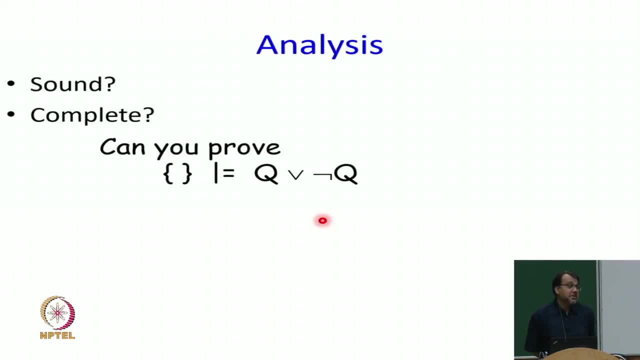 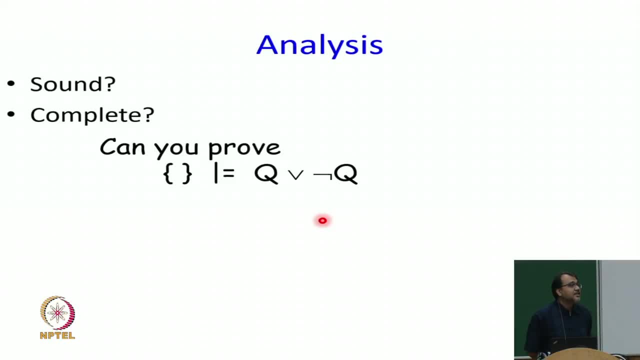 to prove it? No, because forward-chaining only applies modus ponens and this rule. this cannot be proved by modus ponens. However, we know that if kB only has horn clauses and query is a single literal, then forward checking is also complete. Here is the importance of horn clauses And in 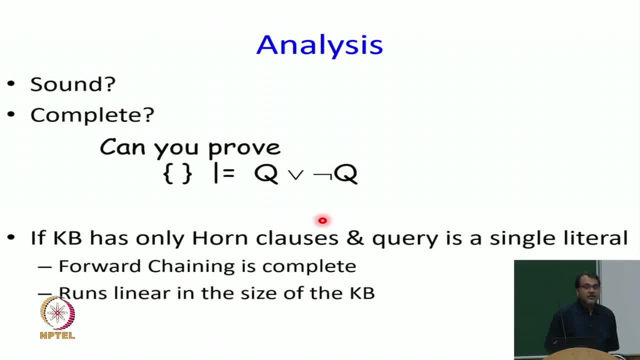 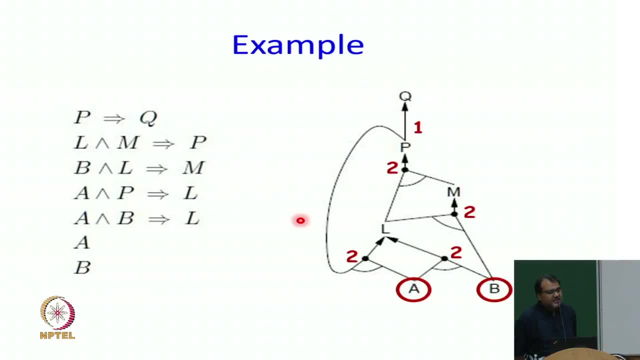 fact, not only is it complete, it runs linear in the size of the knowledge base. Let us look at this example, And I think that will be the last thing we will do today. So suppose these are the things I know in my knowledge base. P implies Q and L and M. 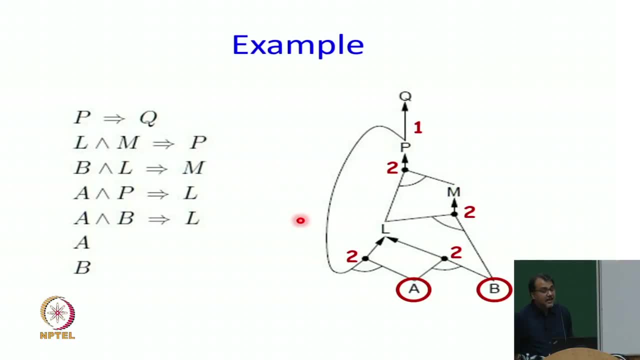 implies P, B and L implies M, A and P implies L A and B implies L. A is true, B is true, And now I ask the question: is Q true? So what I can do is I can convert this particular. 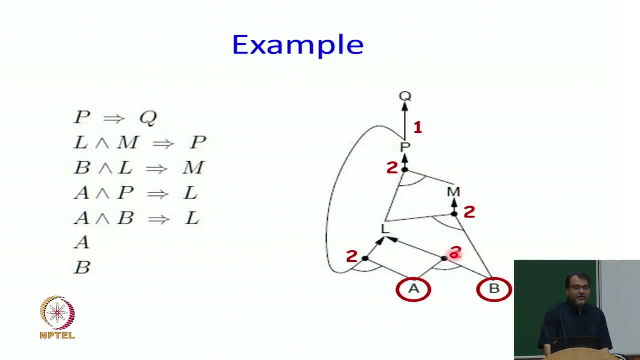 knowledge base into a graph. So here every node is a variable, a proposition. Then I also know that A and B implies L. So the way I represent it is: I take it A and arc out from A and arc out from B and put it in this intermediate node. 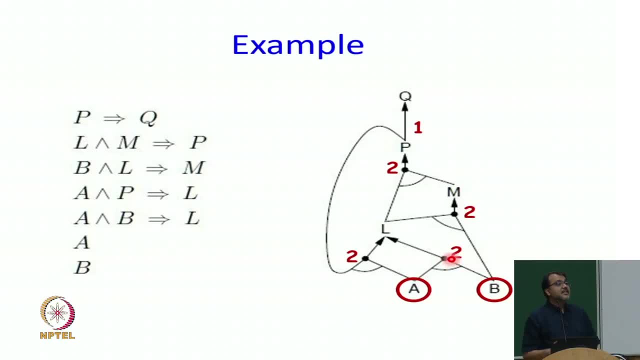 And I make an arc which says: two of these things need to be true for me to get to L, and I make an arc from this dot to the to L. So basically what I am doing, I am keeping track of how many incident variables do I have in the antecedent? antecedent is A and. 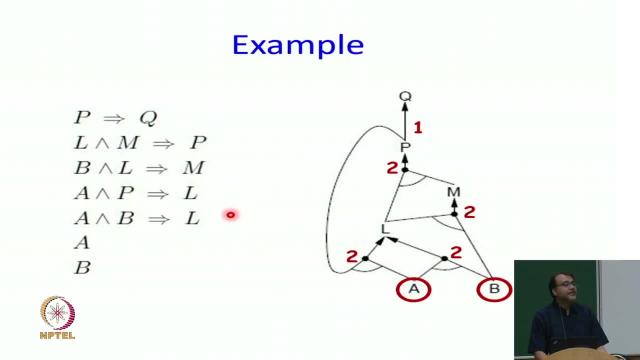 B And what can I prove from it? That is the consequent, And I create this graph structure. And now what I do? I put A and B in my queue because those are the two things I know to be true. Now I can run a simple forward checking algorithm. 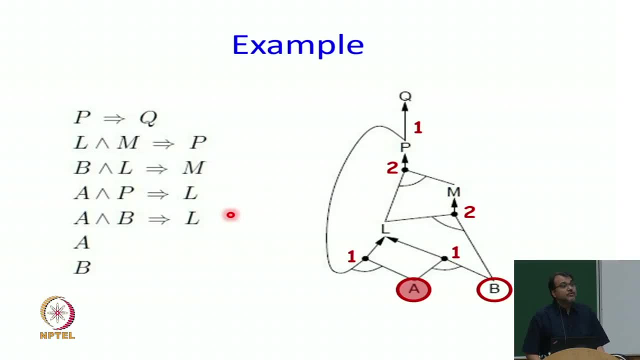 How can I run a simple forward checking algorithm? because A is true, I pop it out from the queue And what do I do from there? as soon as I know A is true, I know that the dot for A and B, the node for A and B, no longer needs two things to be true. it only needs one more. 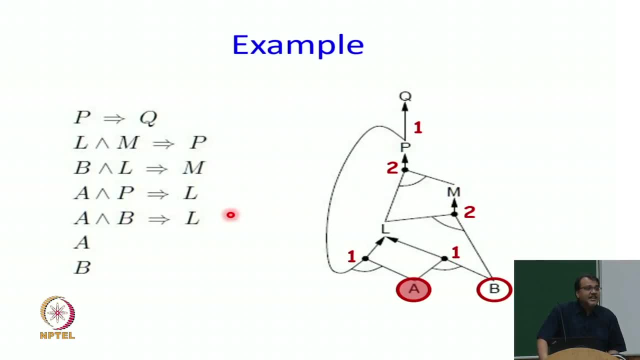 thing to be true. So the antecedent has already got one thing satisfied. Then I pop B, and as soon as I pop B, now I know that I do not need to satisfy: both the things of this antecedent are satisfied, Because both the things of this antecedent are satisfied. 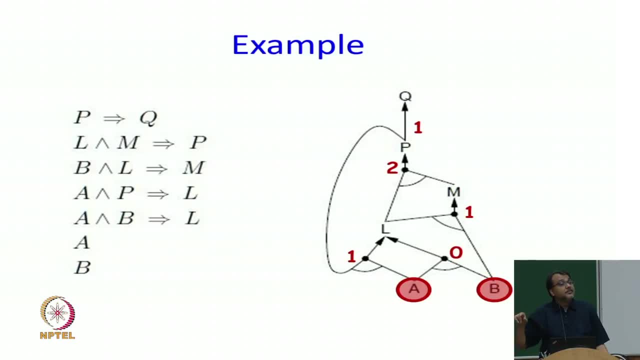 Now I can prove L. because I can prove L, I put it in the queue And I repeat this process. So now that I know L, I have put it in the queue, I pop it from the queue and now I send the messages out saying I have been proven. now you check for yourself.